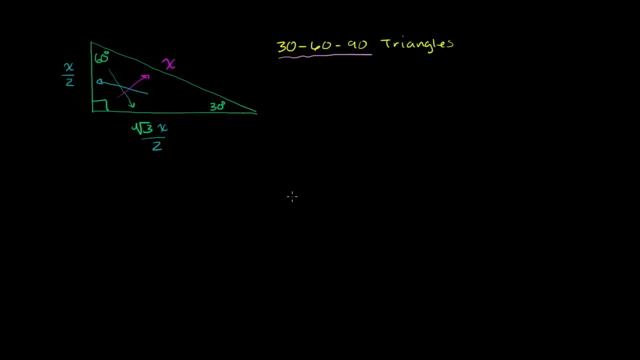 a pretty useful result. Now let's start with a triangle that we're very familiar with, So let me draw ourselves an equilateral triangle. So drawing the triangles is always the hard part, So this is my best shot at an equilateral triangle. 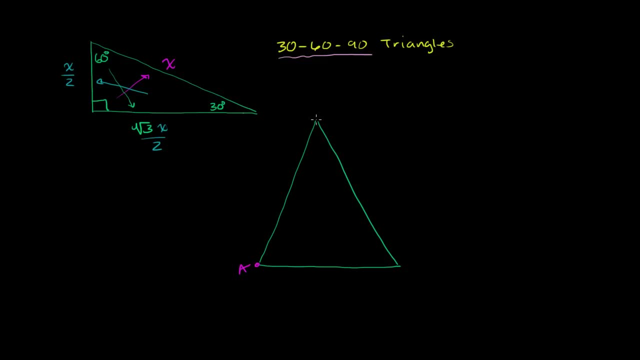 And let's call this ABC. I'm just going to assume that I've constructed an equilateral triangle, So triangle ABC. So triangle ABC is equilateral. And if it's equilateral, that means all of its sides are equal, And let's say that it has length. 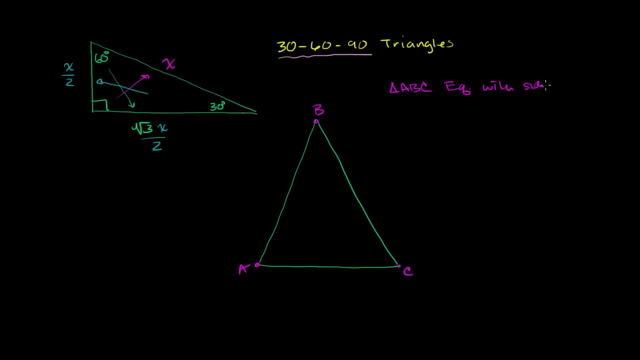 And let's say equilateral, with sides of length x. So this is going to be x, This is going to be x And this is going to be x. We also know, based on what we've seen from equilateral triangles before: 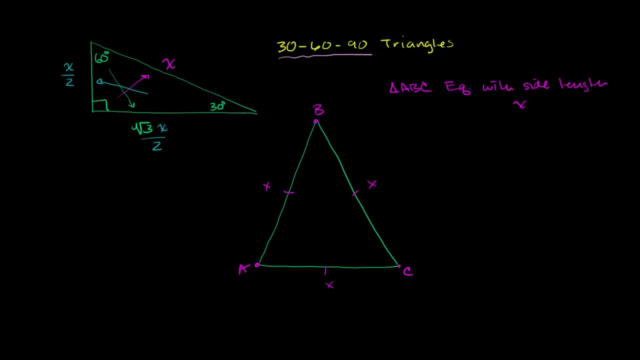 that the measures of all of these angles are going to be 60 degrees. So this is going to be 60 degrees, This is going to be 60 degrees, And then this is going to be 60 degrees. Now, what I'm going to do is I'm going 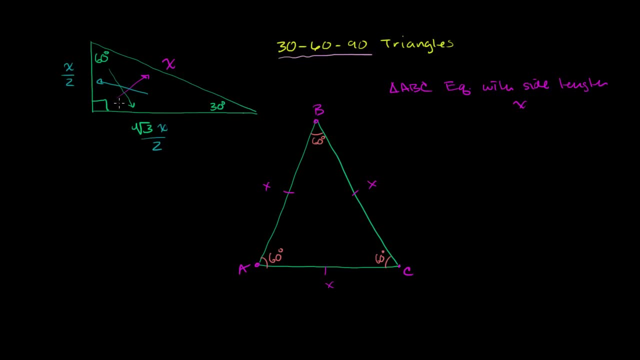 to drop an altitude from this top point right over here. So I'm going to drop an altitude right down And, by definition, when I'm constructing an altitude, it's going to intersect the base right here at a right angle. So that's going to be a right angle. 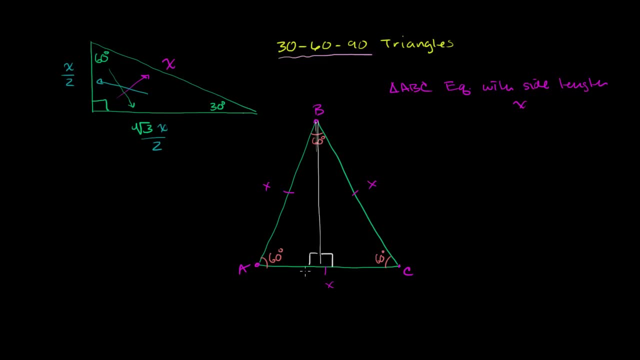 And then this is going to be a right angle, And it's a pretty straightforward proof to show that not only is this an altitude, not only is it perpendicular to this base, but it's a pretty straightforward proof to show that it bisects the base. 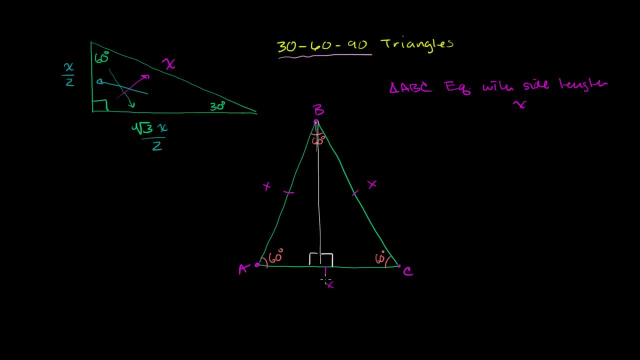 And you could pause it if you like and prove it yourself. But it really comes out of the fact that it's easy to prove that these two triangles are congruent, So let me prove it for you. So let's call this point D right over here. 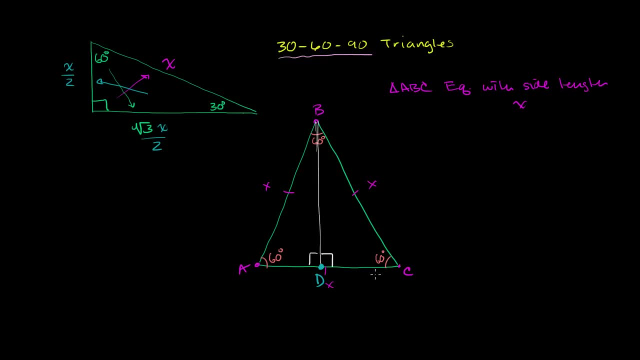 So triangles, ABD and BDC- they clearly both share this side, So this side is common to both of them right over here, And then we could do whatever we have. This angle right over here is congruent to this angle over there. 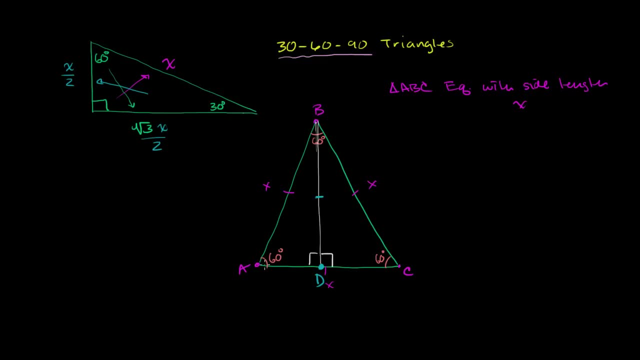 This angle right over here is congruent to this angle over here, And so if these two are congruent to each other, then the third angle has to be congruent to each other. So this angle right over here needs to be congruent to that angle right over there. 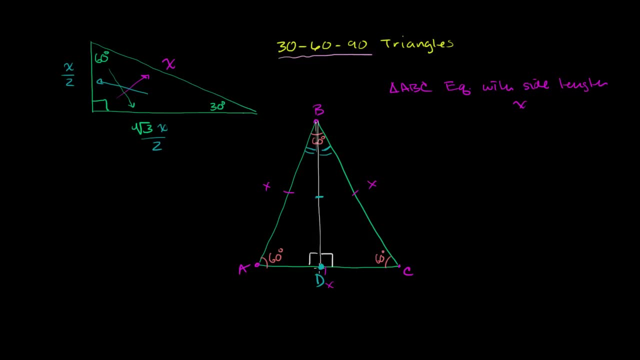 So these two are congruent And so you can use actually a variety of our congruence postulates. We could say side-angle-side, side-angle-side congruence, We could use angle side angle, any of those. 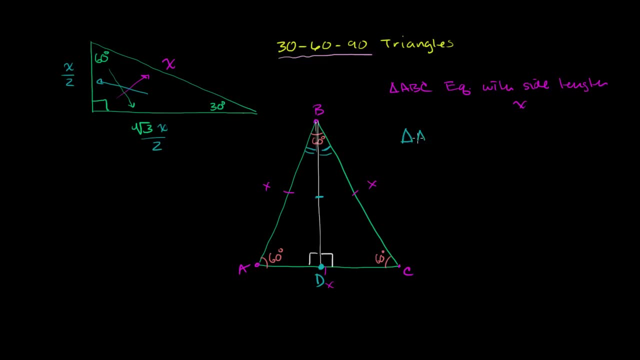 to show that triangle ABD is congruent to triangle CBD And what that does for us and we could use, as I said, we could use angle side angle or side angle side, whatever we like to use for this- what that does for us. 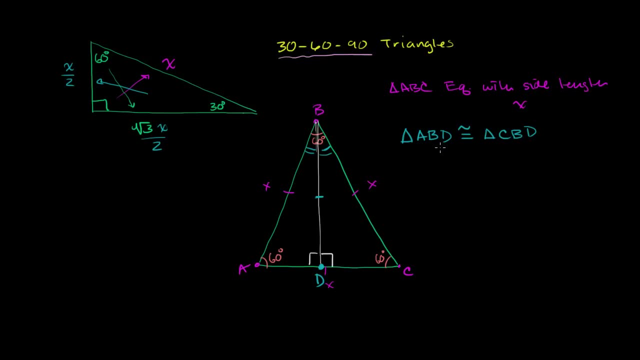 is. it tells us that the corresponding sides of these triangles are going to be equal. In particular, AD is going to be equal to CD. These are corresponding sides, So these are going to be equal to each other. And if we know that they're equal to each other, 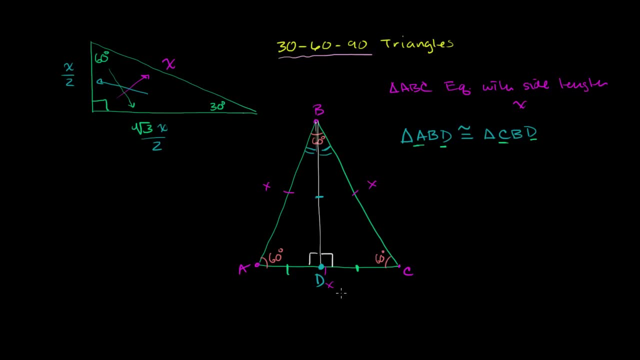 and they add up to x. remember this was an equilateral triangle of length x. we know that this side right over here is going to be x over 2.. Not only do we know that, but we also knew when we dropped this altitude. 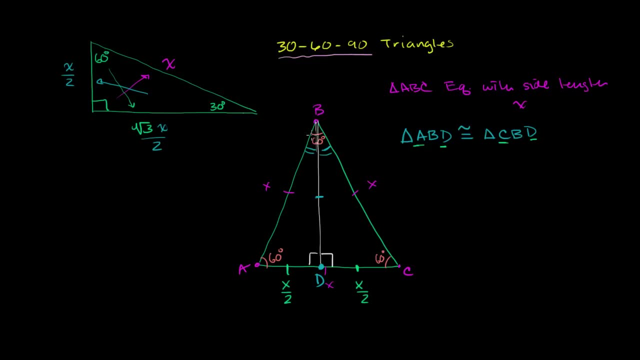 we showed that this angle has to be congruent to that angle and their measures have to add up to 60. So if two things are the same and they add up to 60, this is going to be at 30 degrees and this is going to be 30 degrees. 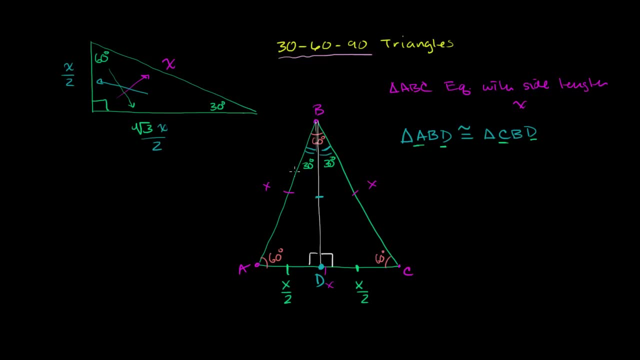 So we've already shown one of the interesting parts of a 30-60-90 triangle that, if the hypotenuse notice- and I guess I didn't point this out- by dropping this altitude I've essentially split this equilateral triangle into two 30-60-90 triangles. 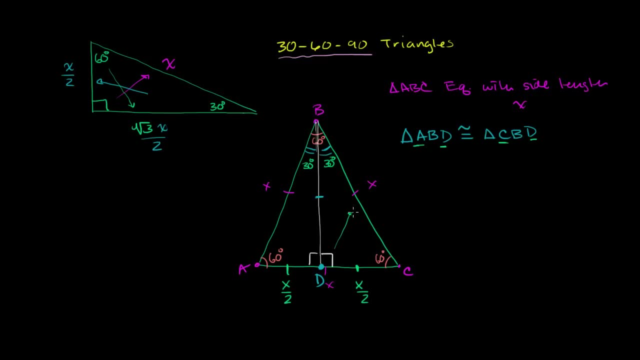 And so we've already shown that if the side opposite the 90 degree side is x, that the side opposite the 90 degree side is going to be x over 2.. That's what we showed right over here. Now we just have to come up with the third side. 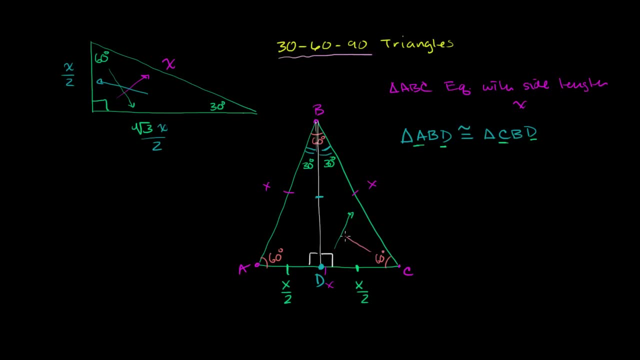 the side that is opposite, the 60 degree side, right over there, And let's call that length. I'll just use the letters that we already have here. This is BD And we can just use the Pythagorean theorem right here: BD squared plus this length right over here, squared. 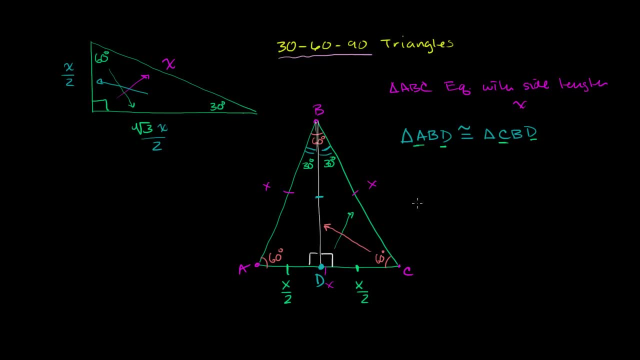 plus x over 2 squared is going to be equal to the hypotenuse squared. So we get BD squared plus x over 2 squared. This is just straight out of the Pythagorean theorem: Plus x over 2 squared is going to equal this hypotenuse squared.